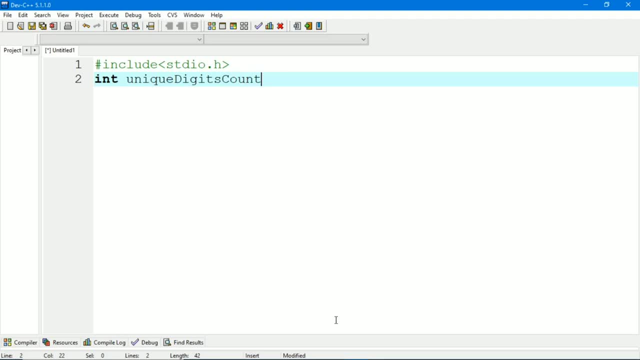 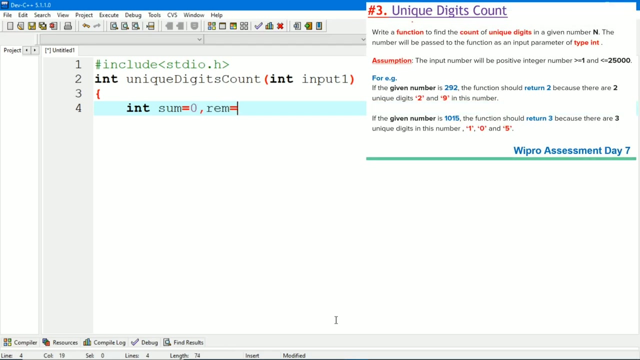 Now we will pass the formal argument as an input, Let's say input 1.. After that, we will initialize some variables. Let's say sum equal to 0 and rem, that is, remainder equal to 0 and count equal to 0.. After that, according to the question here in question, given that input should be greater, 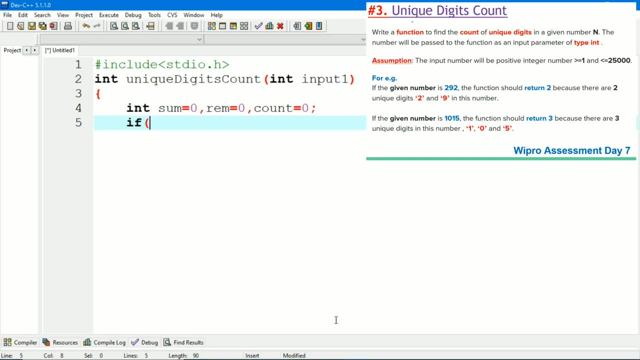 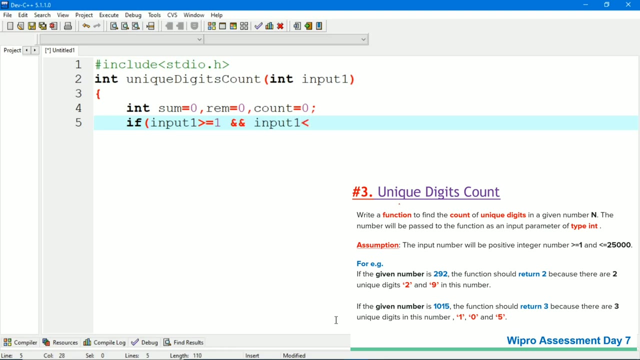 than or equal to 1 and less than or equal to 25000.. So input 1 should be greater than or equal to 1 and input 1 should be less than or equal to 25000.. After that, we will declare and initialize one error which contains pain element. all, all of the. 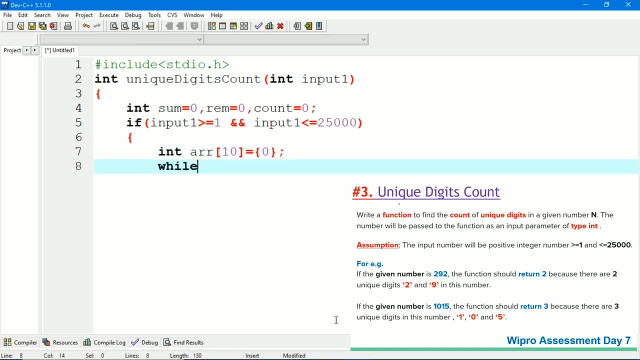 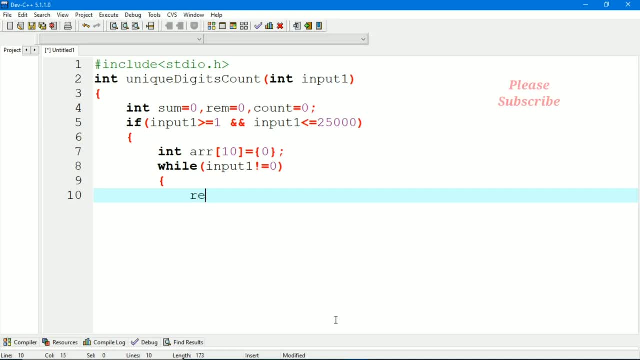 element is 0. Now, while input 1 is not equal to 0, we will continue the loop. Then remainder equal to equal to input 1, modulus 1.. And if if a error of remainder equal to equal to 0, we will do the error of remainder to 1.. 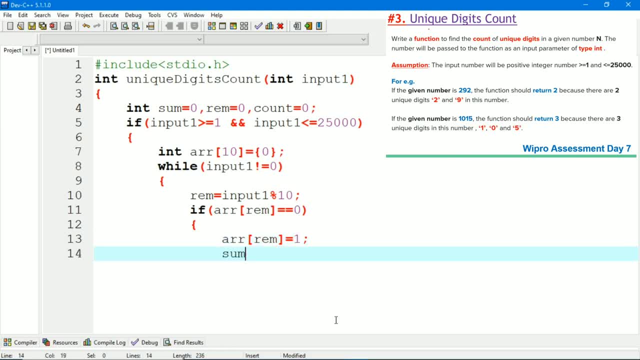 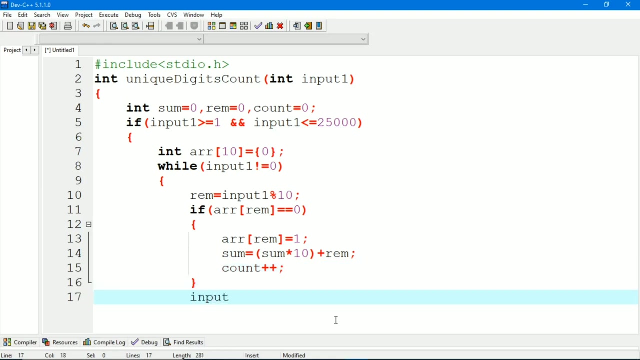 After that: sum equal to sum into 10.. Let's say 0 is equal to 0 and remember we will start from 0 and remember we will count now, count plus plus. After that: input 1 equal to input1 divided by 10.. 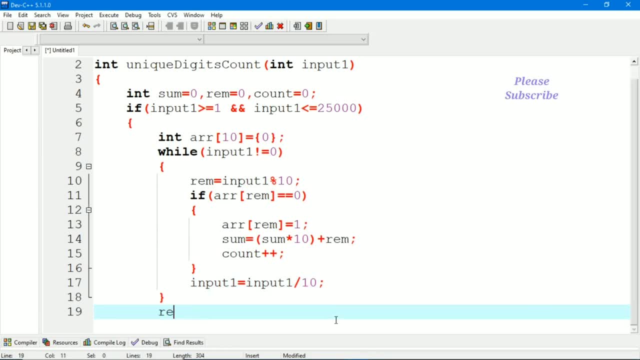 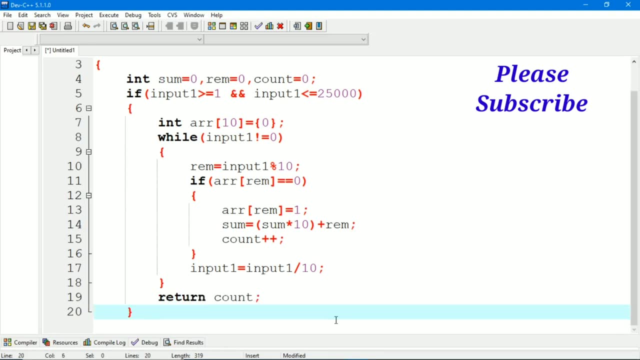 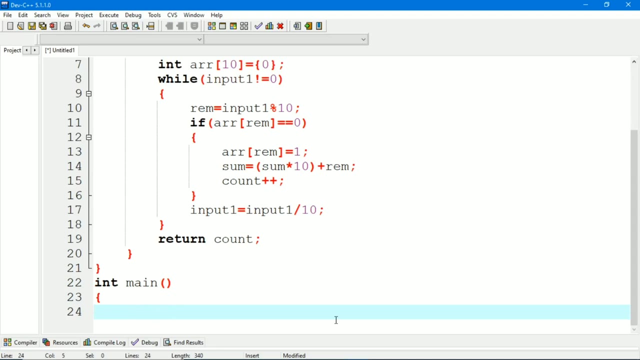 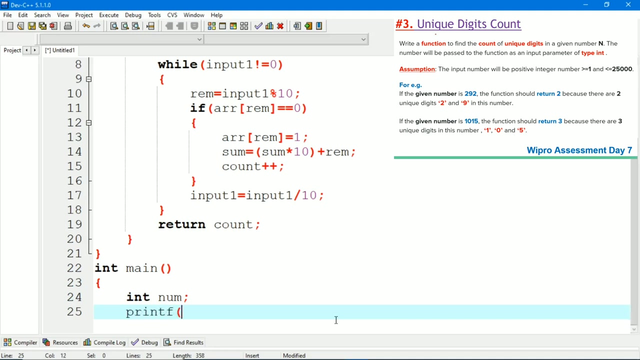 Now return count, We will get counter input 2 and we will write 10.. We will write 10.. We will write 10.. Now we will write the main function, int main, and we will take one input variable, that is number. now we will take the input from user. now enter the number and we will read it from. 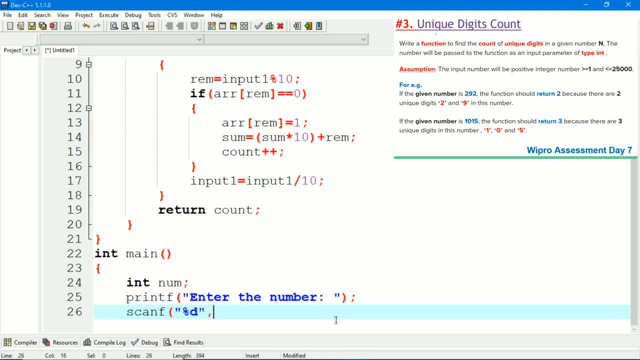 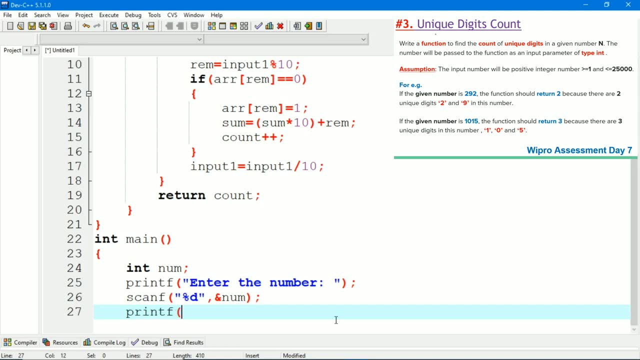 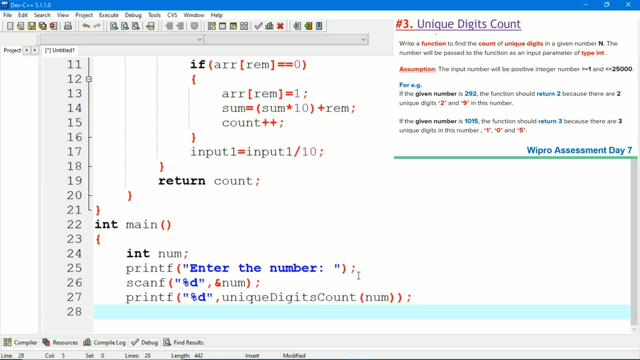 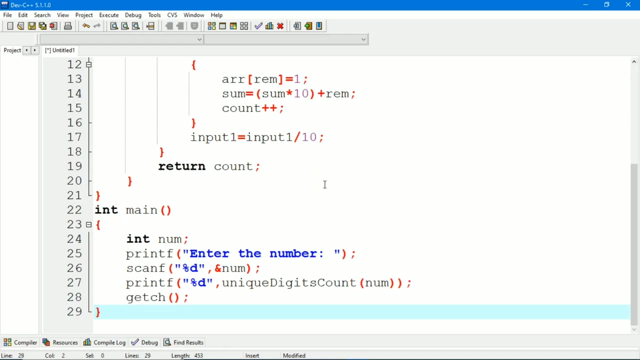 keyboard %d &% number and now we will call the function %d. here our function name is unique digits count. so here we will write unique digits count and we will pass the function number variable at last. gets yes, for hold the screen now by pressing ctrl s, we will. 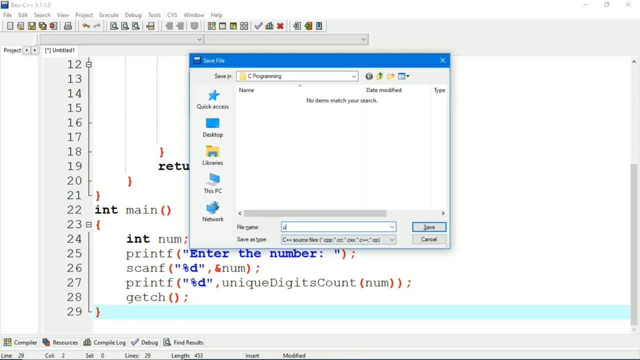 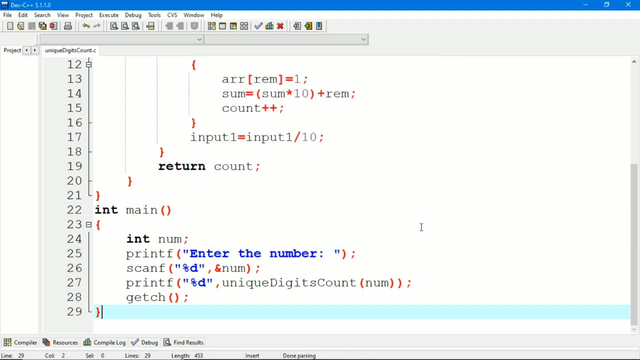 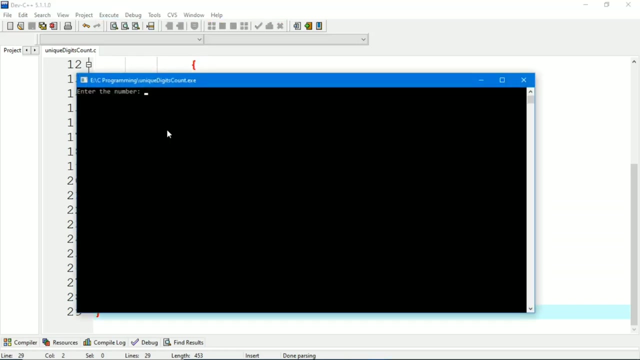 save the program. let's name as: unique digits: count. unique digits: countc. now we will select the all files. let's save. Now we will run the program. Now we will execute the program: execute, compile and run. let's give the input as 292. here our 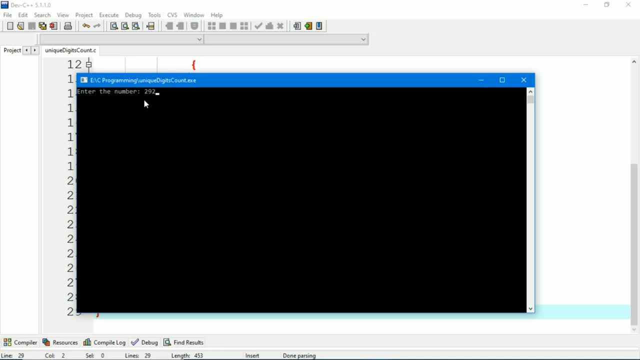 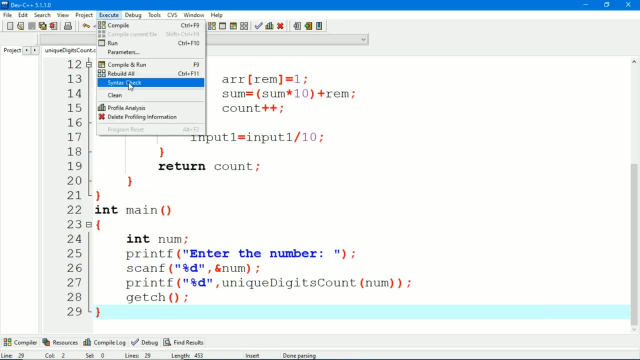 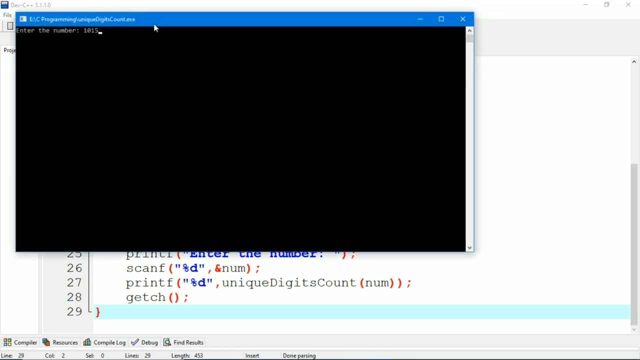 program should return 2, because there are two unique digits in 292, that is 2 and 9. press enter: here we can see that our program returns 2. now let's check for another input. Let's say 1015. here we can see that there are 3 unique digits, that is, 10 and 5. so our 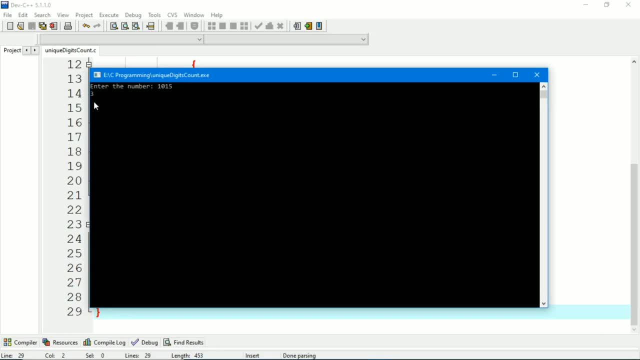 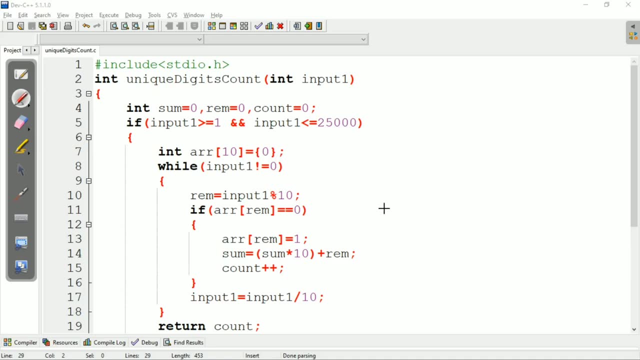 program should return 3. here we can see that it returns 3, so our program is right. now we will see how it works. at first we have taken one formal argument as an input, that is input 1.. Now we will see how it works. 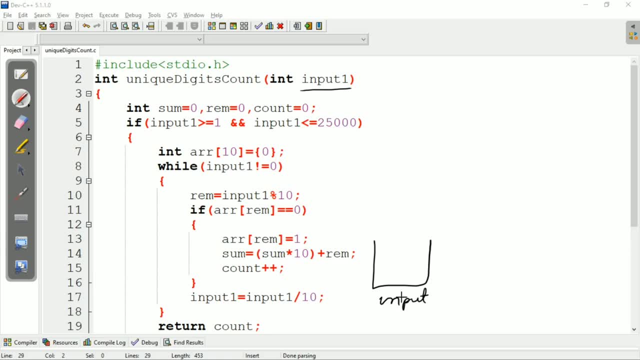 At first we have taken one formal argument as an input, that is input 1.. We will take one input, let's say 292. we will check how many unique digits are present in 292. after that we have initialized some variables. that is, sum equal to 0, sum equal. 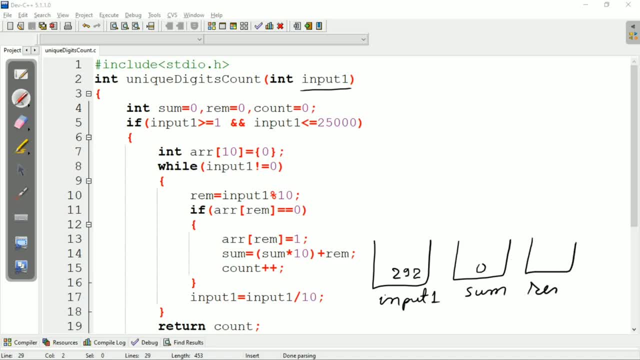 to 0 and reminder equal to 0. And count equal to 0. now, according to question, we are given that input 1 should be greater than or equal to 1 and input 1 should be less than or equal to 25000. after that we have: 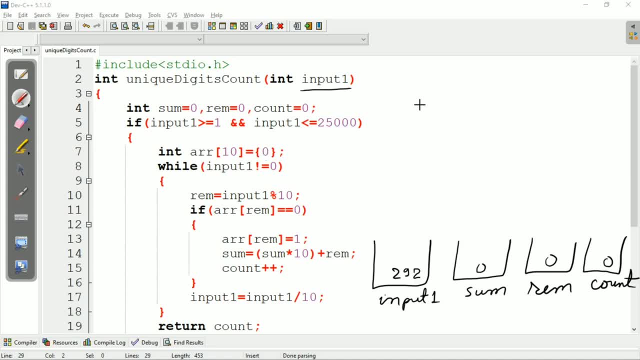 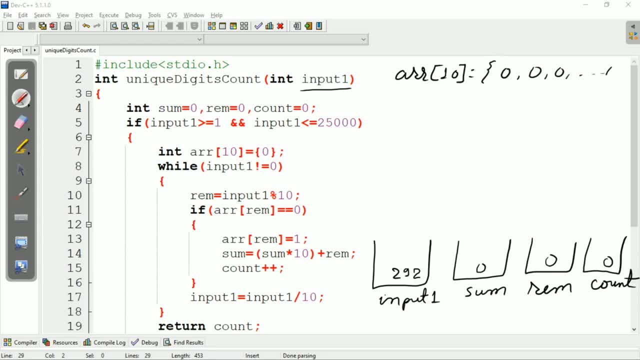 Which consists of all the zero element. Let's say index 0, 1, 2, 3, 4, 5, 6, 7, 8.. Let's say: index 0, 1, 2, 3, 4, 5, 6, 7, 8.. 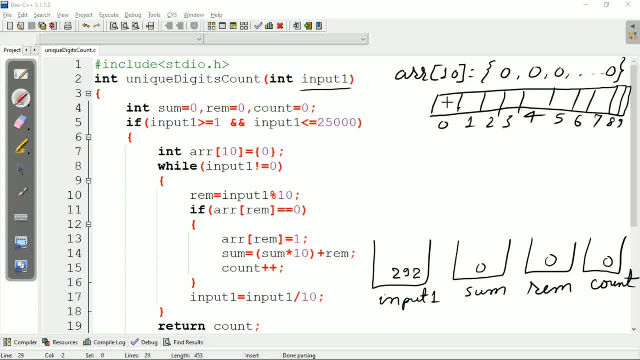 Let's say index 0, 1, 2, 3, 4, 5, 6, 7, 8.. And 9 means 0 to 9.. All consists of value 0.. Now, while input 1 is not equal to 0, here we can see that 292, which is not equal to 0. 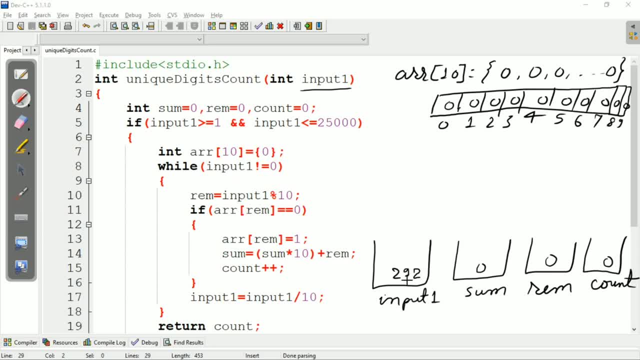 So reminder equal to input 1, modulus 10.. So 292 modulus 10 equal to 2.. Here reminder becomes 2.. After that, if ARR of reminder Equal to equal to 0 means ARR of 2, here reminder equal to 2.. 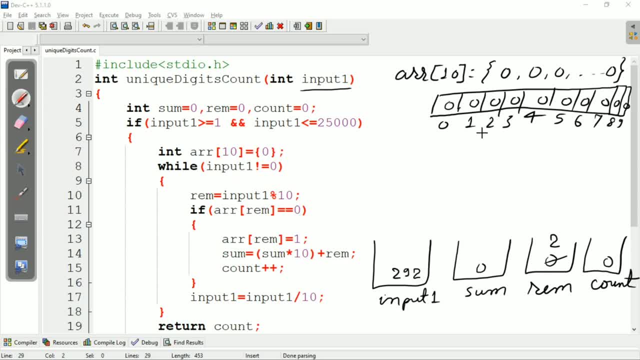 So ARR of 2 equal to equal to 0. We can see that ARR of 2 equal to 0. So ARR of remainder equal to 1.. So remainder becomes means value in the ARR of remainder becomes 1.. So here 0 is updated to 1.. 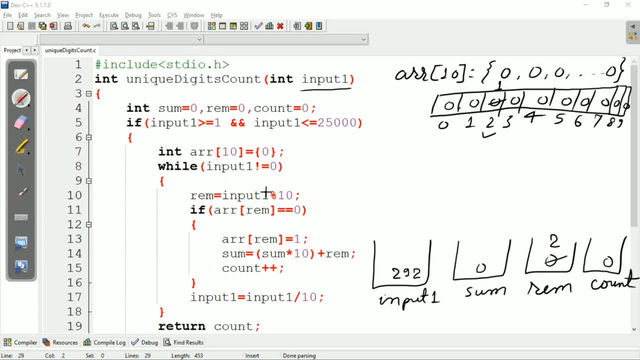 After that: sum equal to sum into 10 plus remainder. Here initially sum equal to 0. So sum into 10 means 0 into 10, plus remainder equal to 2.. So here sum is updated to sum will be updated to 2.. 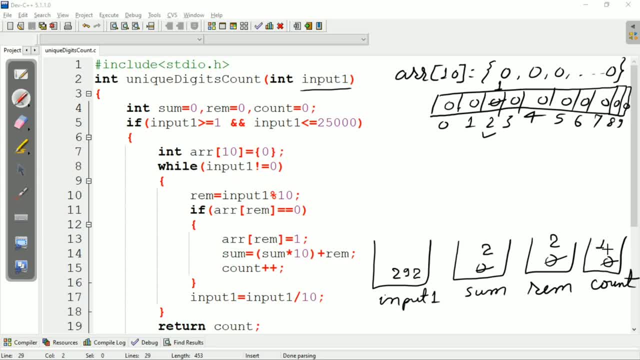 Now count plus plus, So count becomes 1.. Now again input 1 equal to input 1 divided by 10.. So input 1 becomes 29, because 292 divided by 10 is 29.. After that again, input 1 is not equal to 0.. 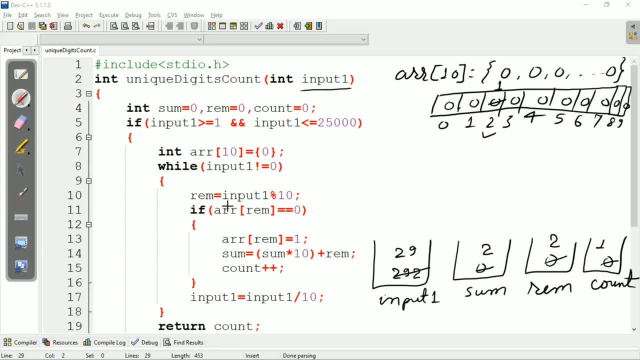 Here we can see that 21.. 29.. 29 is not equal to 0.. So remainder equal to input 1 modulus 10.. So here remainder becomes 29 modulus 10.. So here 9.. Now ARR of remainder equal to equal to 0. 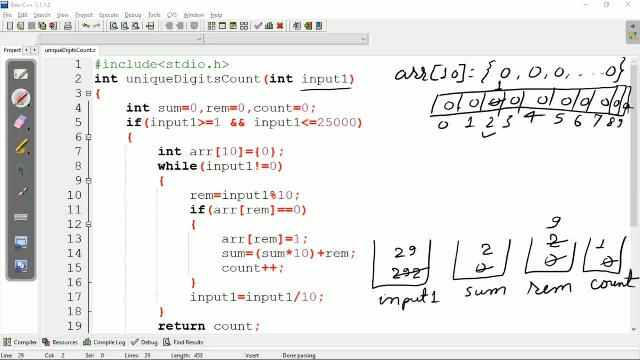 Here we can see that ARR of 9 equal to 0. So condition is true. So ARR of remainder equal to 1. Here 9 means value of the index. 9 becomes 1. So here 1.. Now again, Sum equal to sum into 10 plus remainder. 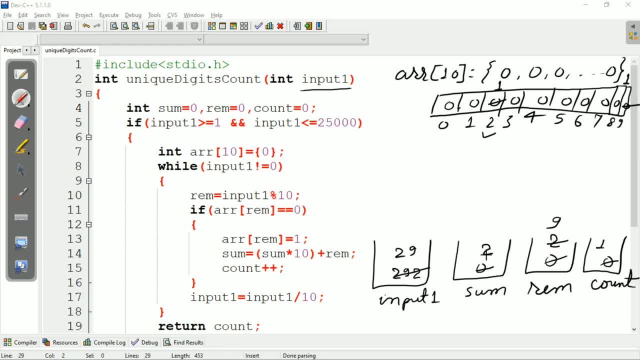 Here sum equal to 2.. 2 into 10.. 20.. 20 plus 9. Here sum becomes 29.. Now again count plus plus. Here count becomes 2.. Now input 1 equal to input 1 divided by 10.. 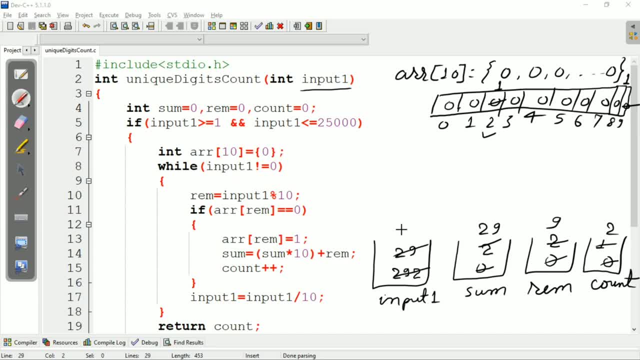 Here 29 divided by 10. Input 1 becomes 2.. Now again we will check the condition. Input 1 is not equal to 0.. Here 2 is not equal to 0. Condition is true, So again, remainder equal to input 1, modulus 10.. 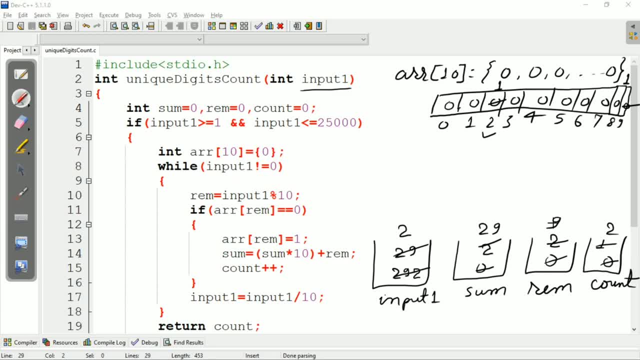 Here remainder equal to input. 1 is to 2 modulus 10.. So remainder becomes again 2.. Now again we will check if ARR of remainder equal to equal to 0. Here ARR of remainder means ARR of 2.. Here we can see that ARR of 2 equal to 0. 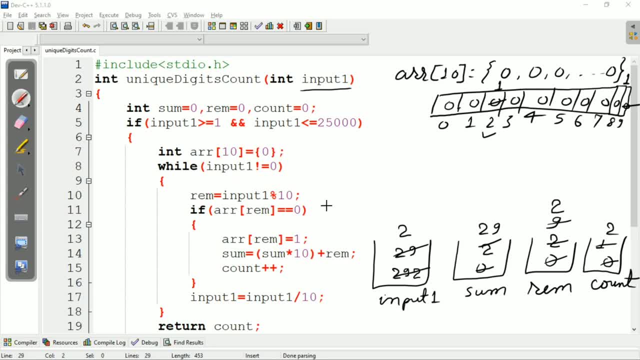 But here condition is ARR of remainder equal to 0. But here 1.. So condition is false. So we will comes out of the loop And again input 1 equal to input 1 divided by 10.. Here 2 divided by 10.. 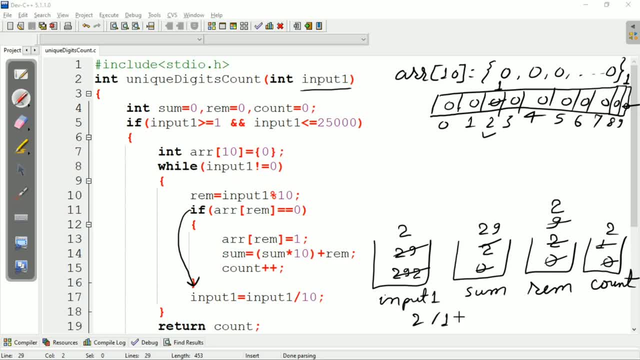 Means 2 divided by 10. It becomes 0. So here input 1 becomes 0.. Now again we will check the condition. While input 1 is not equal to 0. But here input 1 is 0. So condition is false. 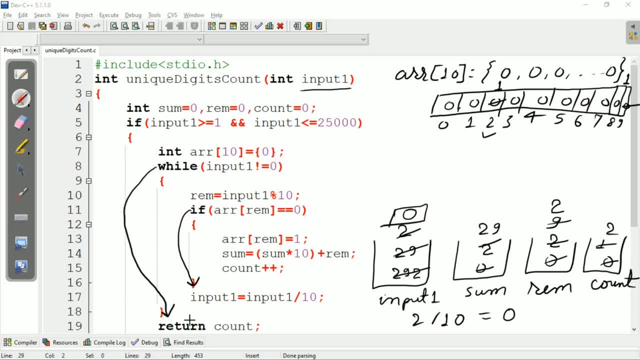 We will comes out of the loop. So after that we will return the count value. Here our count value is 2.. So we know that in 292 the unique digits, total number of unique digits, is 2.. So our program returns 2.. 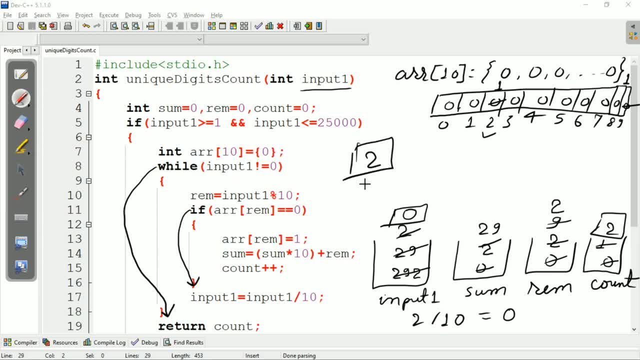 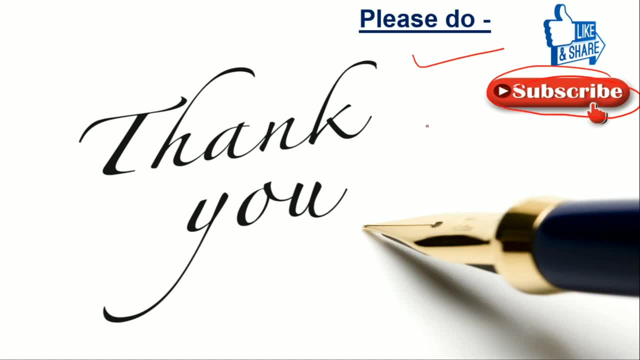 So it will be the answer. Please do like and share this video And subscribe our channel for more these types of questions and solutions. Thank you for watching. See you next time, Bye. 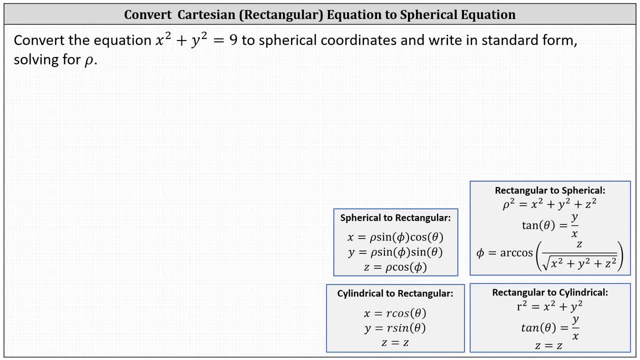 We're asked to convert the Cartesian or rectangular equation x squared plus y squared equals nine to spherical coordinates and write in standard form solving for rho. I'm going to go and show two ways of performing the conversion. Let's begin with the given equation. 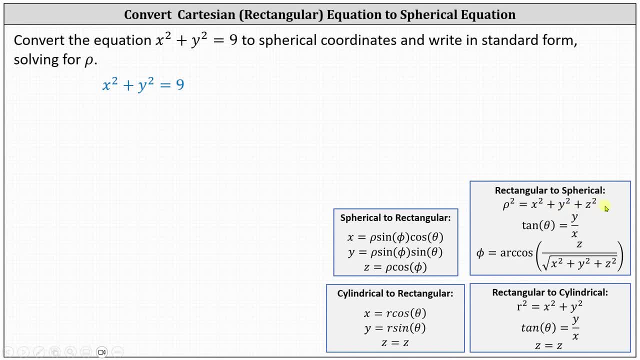 Because rho squared equals x squared plus y squared plus c squared. we can say x squared plus y squared equals rho squared minus c squared. Let's perform this substitution, which gives us rho squared minus c squared equals nine. Next, z equals rho cosine phi. 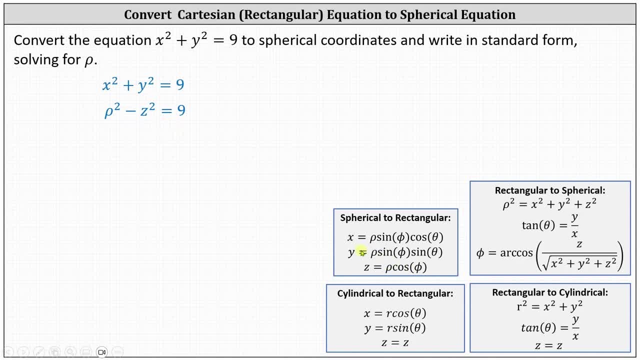 and therefore z squared is equal to rho squared cosine squared phi. So now we have rho squared minus. rho squared cosine squared phi equals nine. Now we'll factor out the greatest common factor on the left of rho squared, which gives us rho squared times the quantity. 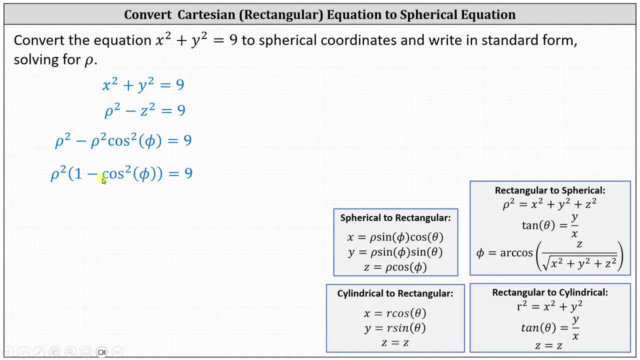 one minus cosine squared phi. Using our trig identities, one minus cosine squared phi equals sine squared phi. Next, we'll divide both sides by sine squared phi, And now we'll take the square root of both sides of the equation. Algebraically, we do have a plus or minus on the right.